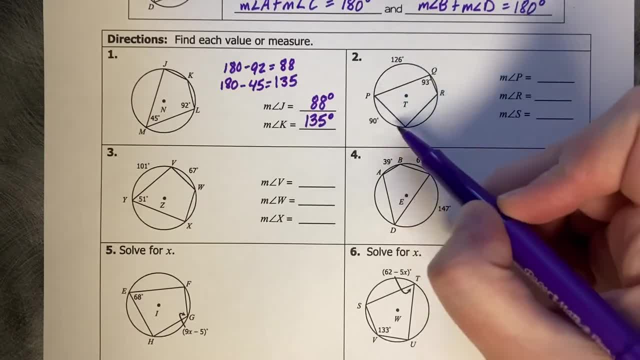 some arc measures on it. So we're going to take a look at number two. So we're going to take a look at number two. So we're going to take a look at number two. So we know this is a 126,, a 90,, 93.. I 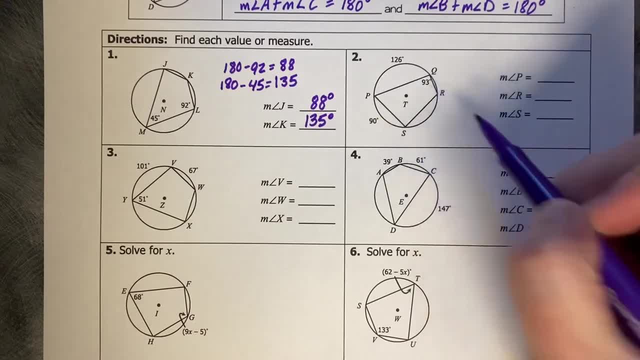 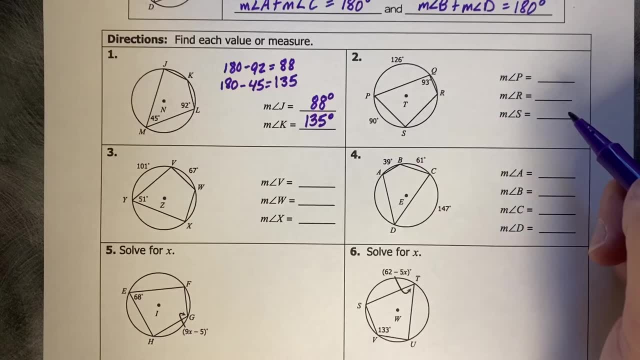 know that's opposite of S, And then we've got P and R opposite of each other as well. So the first one that we could go for is actually angle S. That one's the easiest, I would say, because it's opposite of 93.. So 180 minus 93 is 87.. So angle S is 87 degrees. 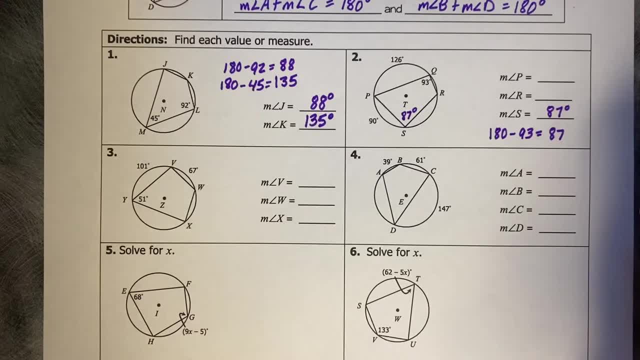 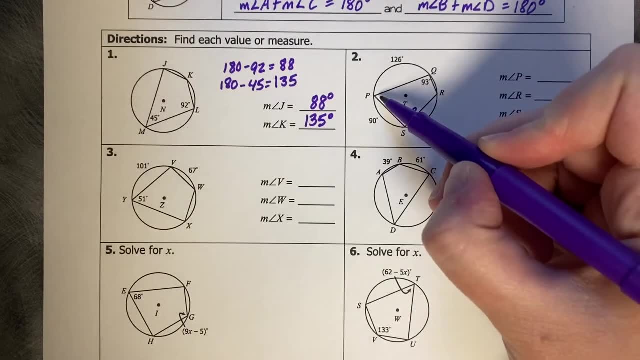 So angle S is 87 degrees. Now here comes some of our knowledge that we have from inscribed angles. So if we'd like to know one of these angles- angle P or angle R- angle R corresponds to- let me use a highlighter to- 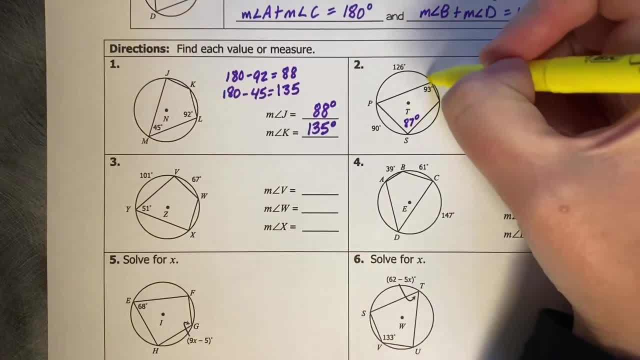 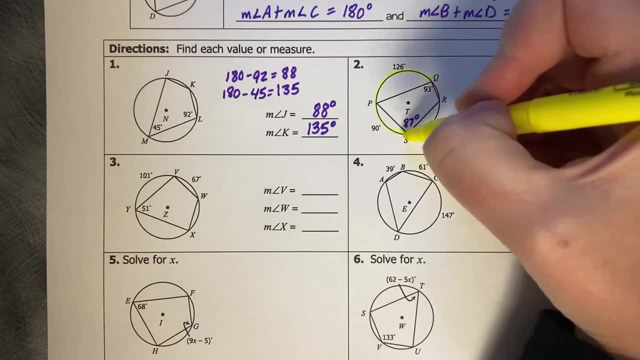 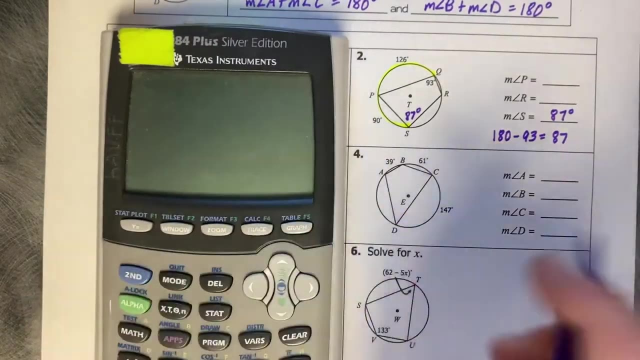 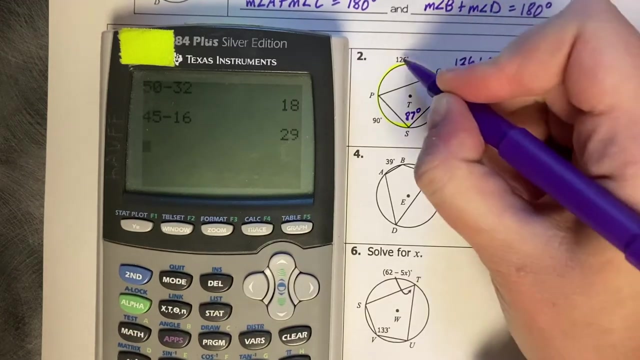 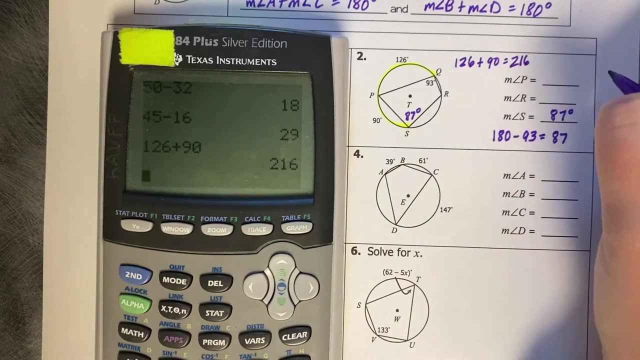 highlight it. Angle R corresponds to this major arc, So that angle R is an inscribed angle inside this circle And that means we can use that to work backwards for our angle measure at angle R. So if we do 126 plus 90, so those two pieces of the arc is 216. Then we divide that in half to get angle R. 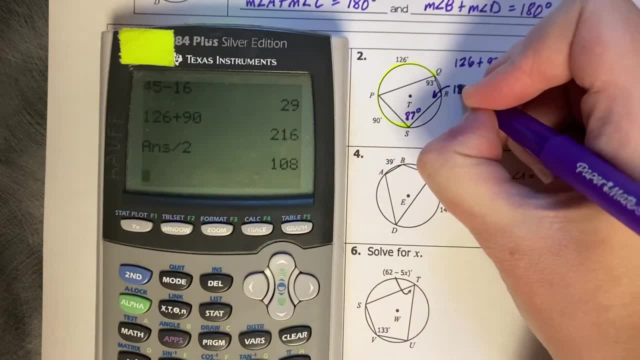 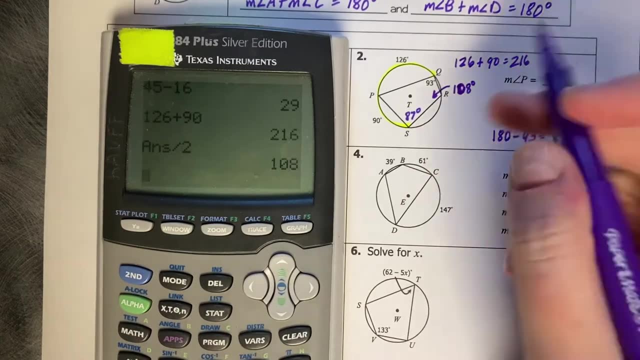 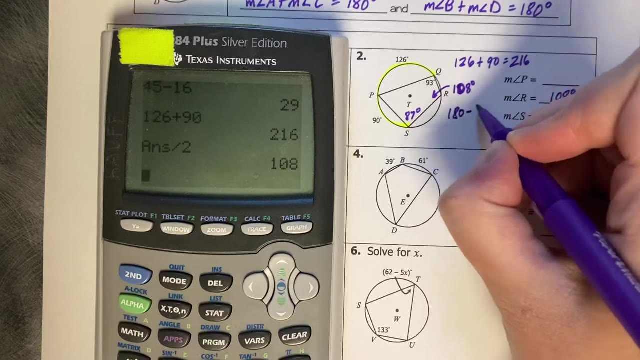 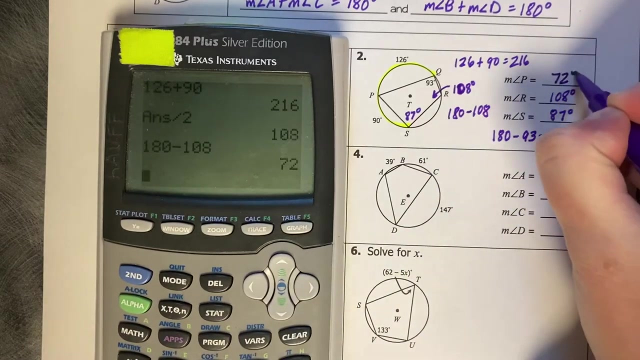 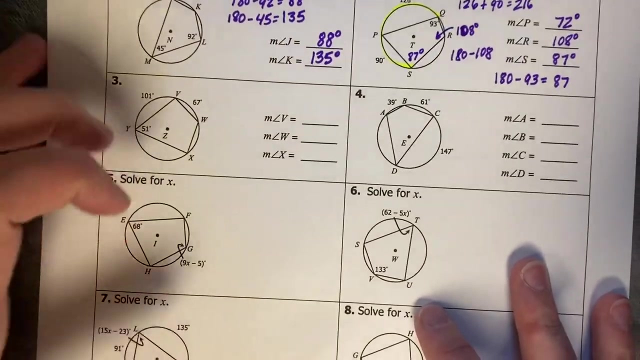 So then angle R is 108, whoops, 108 degrees. And if this is 108 degrees then we can subtract it from 180 to get angle P. So 180 minus 108 is 72 degrees. You go ahead and try number three and four on your own. 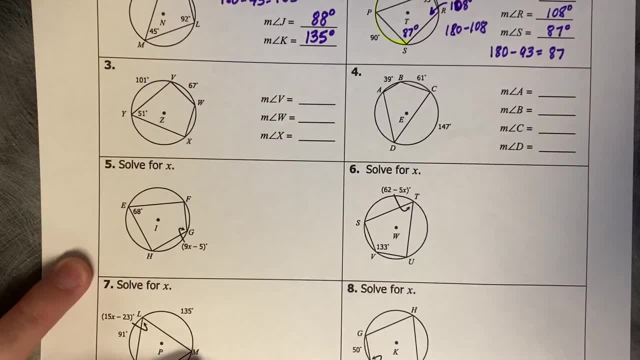 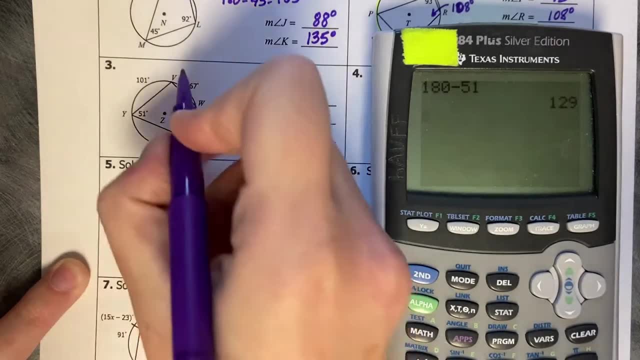 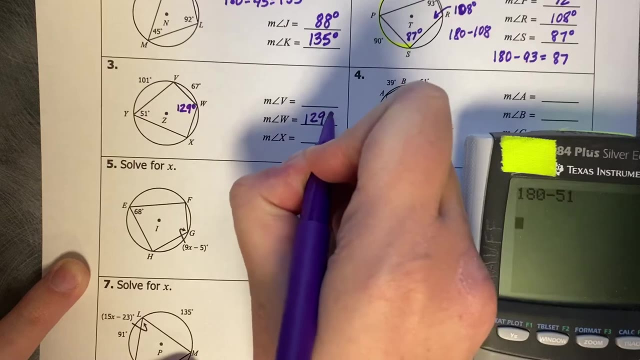 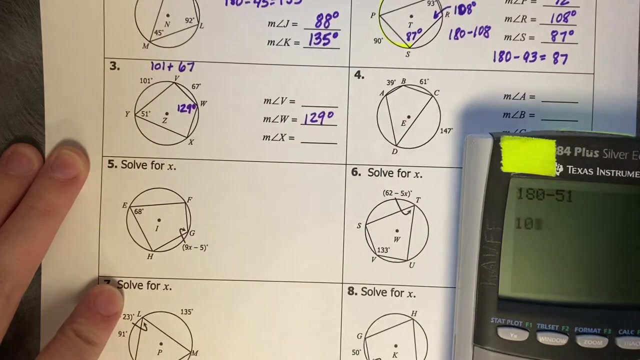 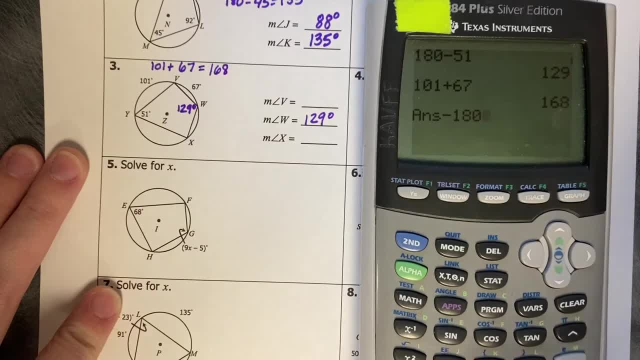 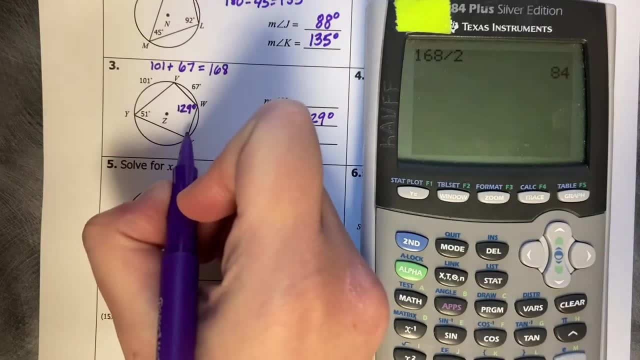 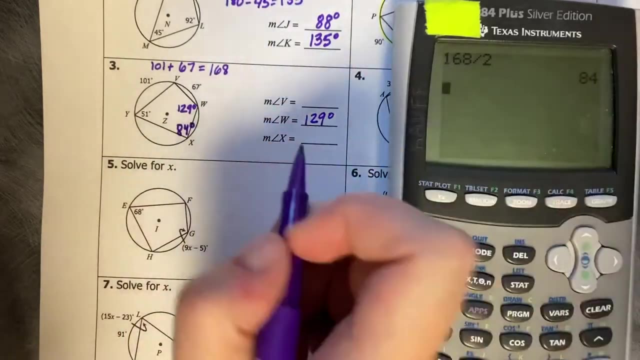 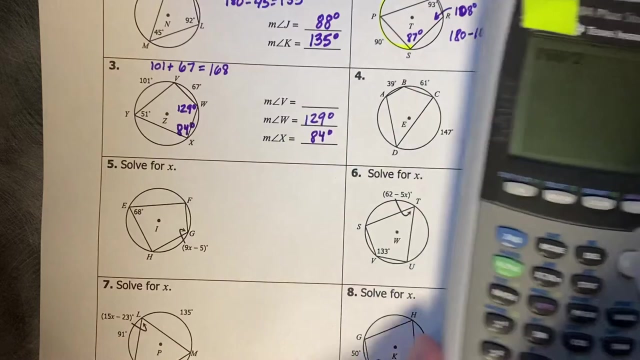 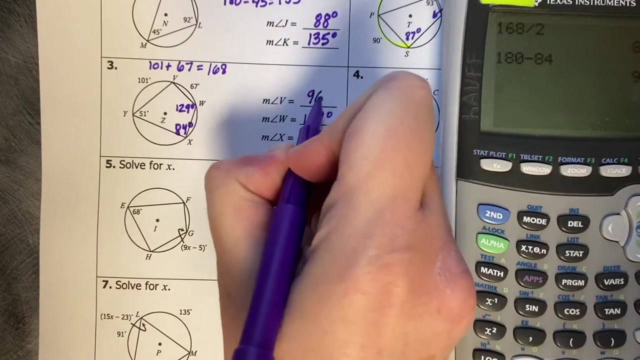 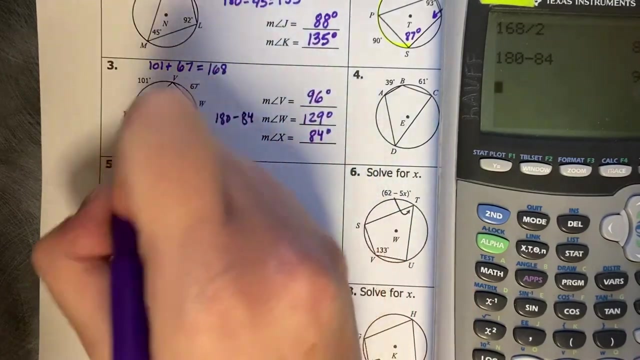 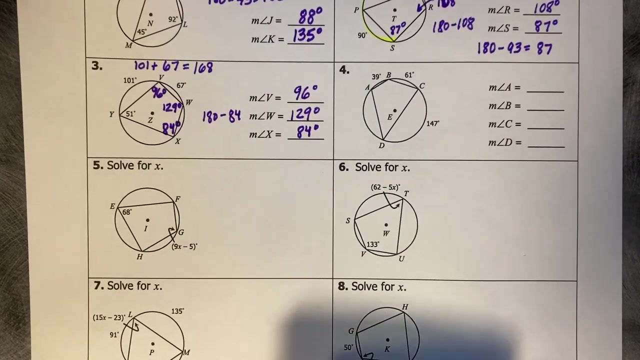 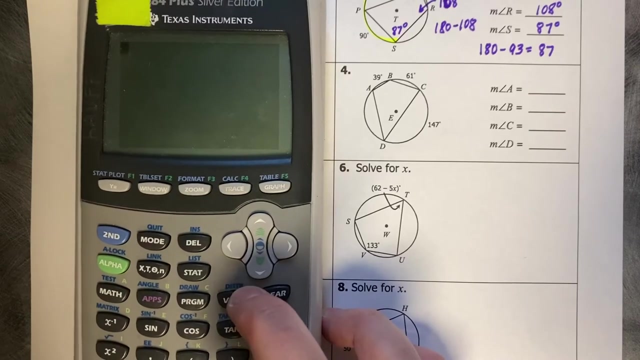 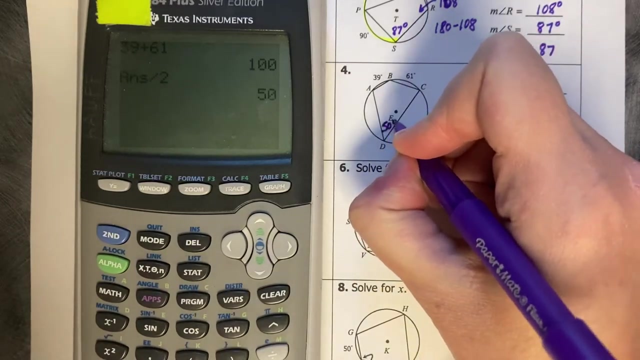 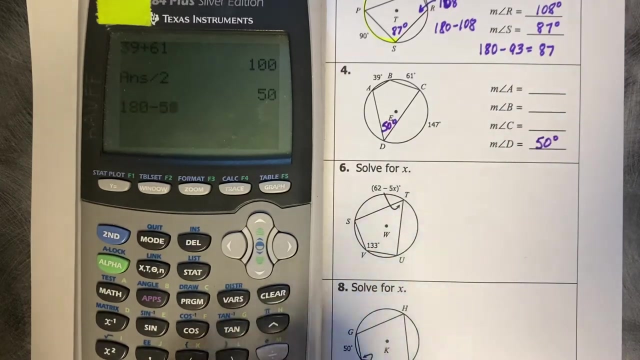 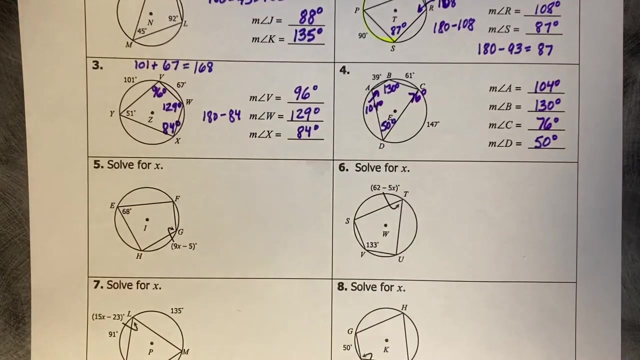 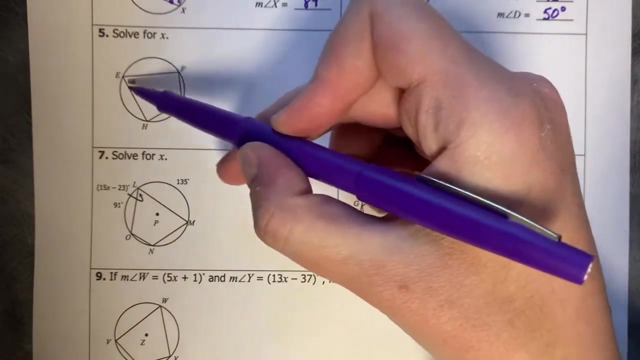 Oops, Oh my God, Oh my God. Okay, let's try some with some variables. Solve for x. So if we know that these two angles are opposite of each other from a quadrilateral, we know that they're supplementary. 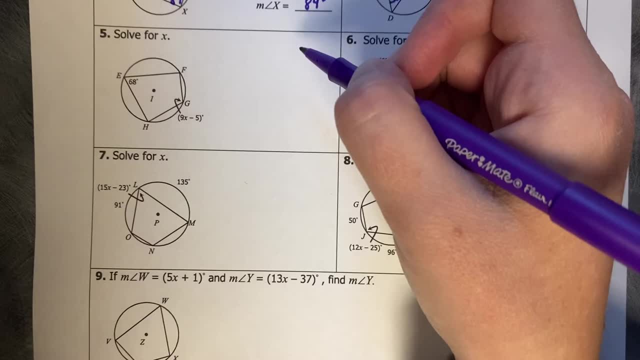 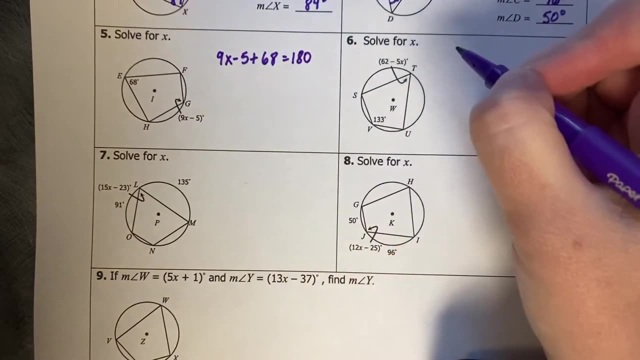 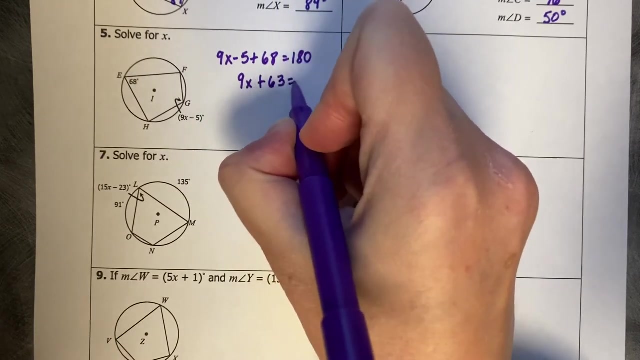 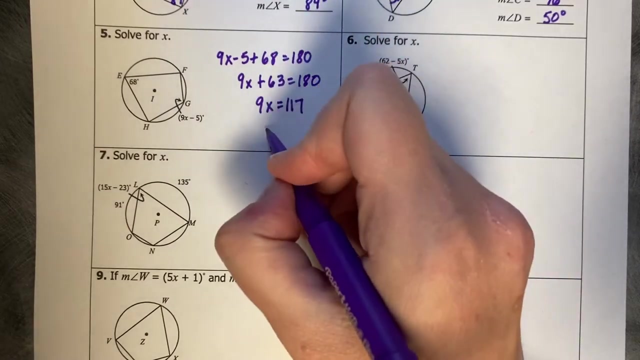 So we can add these two together and set it equal to 180.. So 9x minus 5 plus 16.. 68 equals 180.. 68 minus 5 is 63.. Minus 63,, 117.. Divided by 9, x equals 13.. 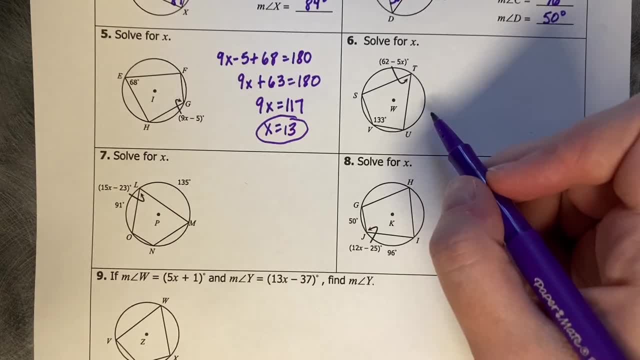 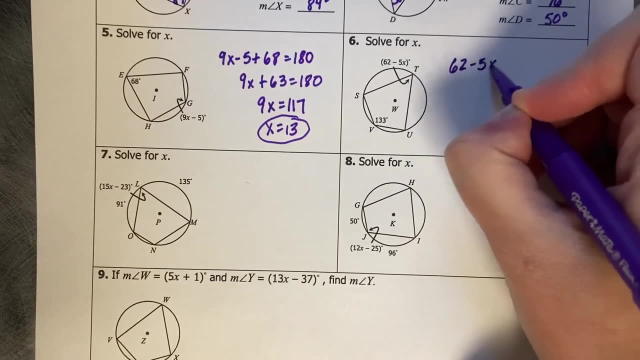 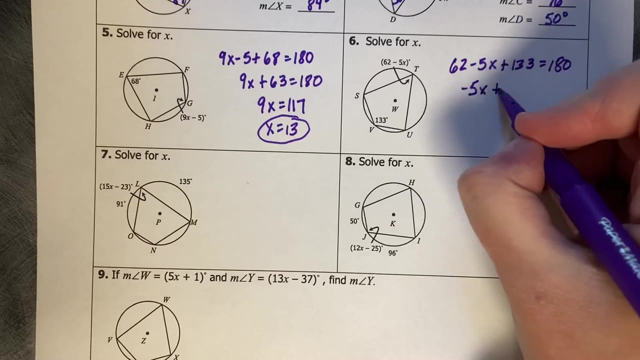 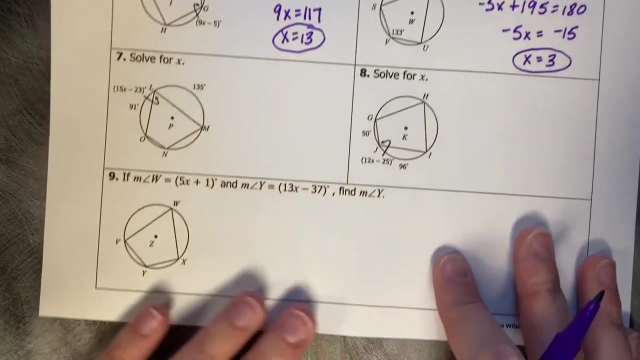 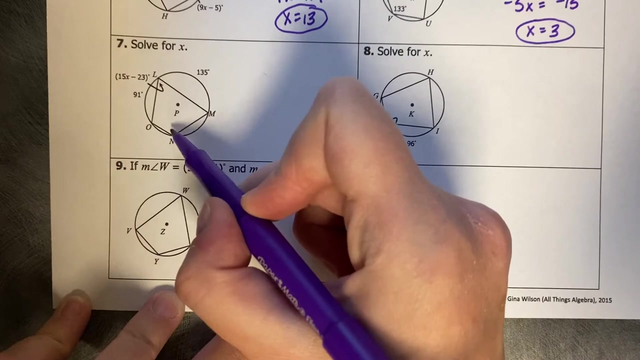 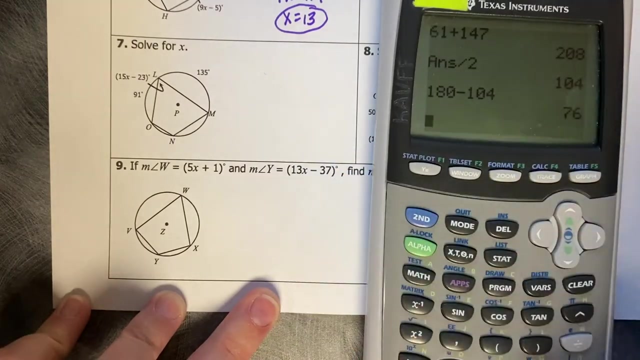 You try number 6 on your own. All right, let's try number 7.. So this one, we're going to have to use our arc measures and this inscribed angle n To be opposite of angle L. So first thing we need to do is add together the 91 and the 135. 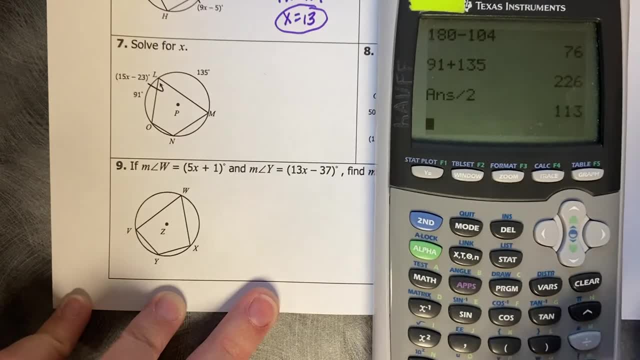 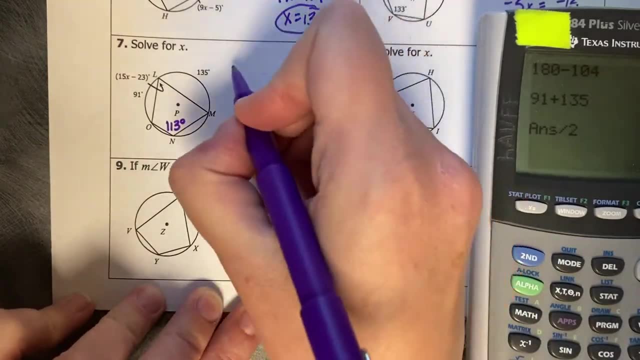 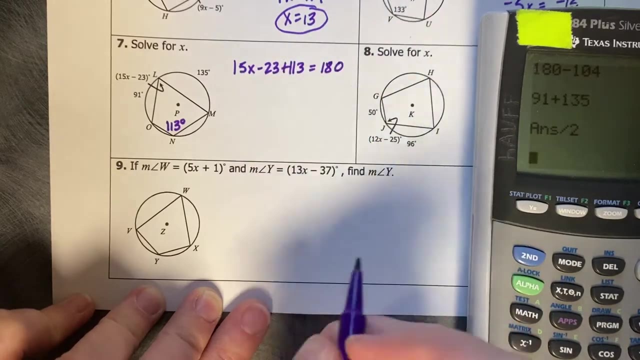 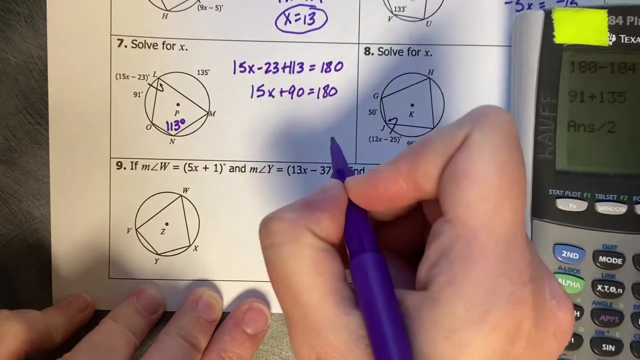 So that's 226 divided by 2 is 113.. For that angle measure n and we can use that to set up our equation. So 15x minus 23 plus 113 equals 180.. Okay, 15x plus 90 equals 180. 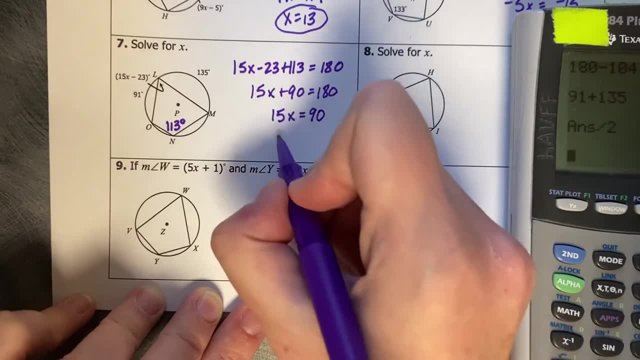 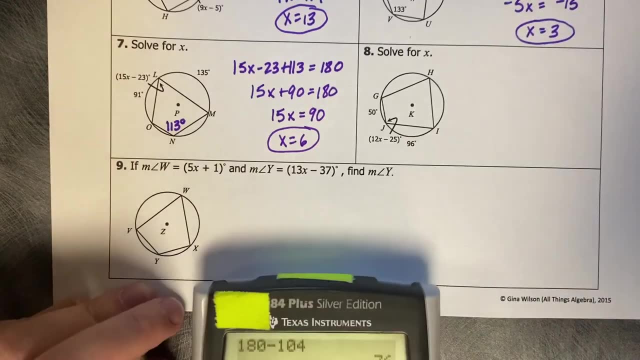 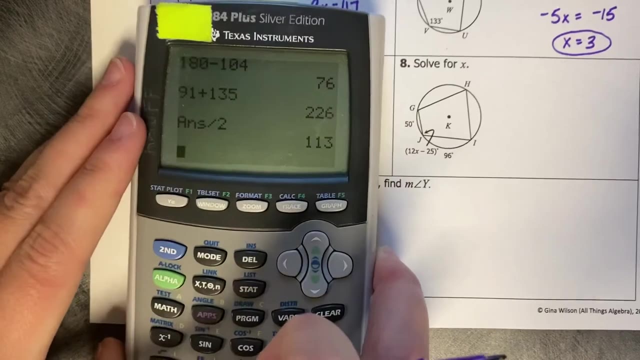 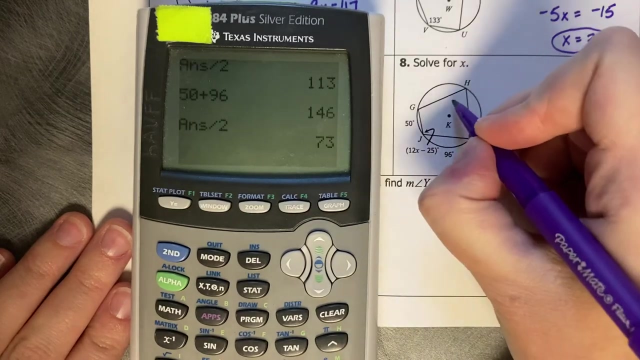 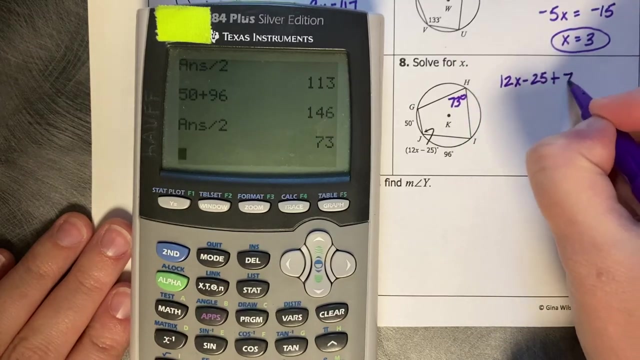 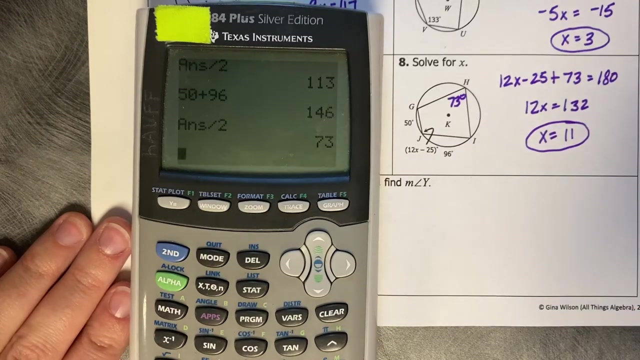 15x equals 90.. nx equals 6.. You try number 8 on your own. So 19,, 215, 139, 그래도 23, 18, 29, 29, 30, 40, 41, 42, 51, All right, last one number nine. 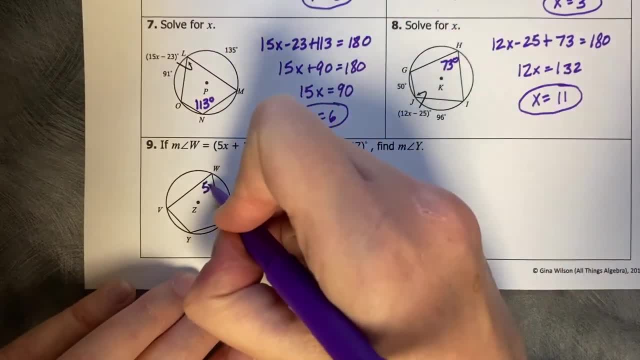 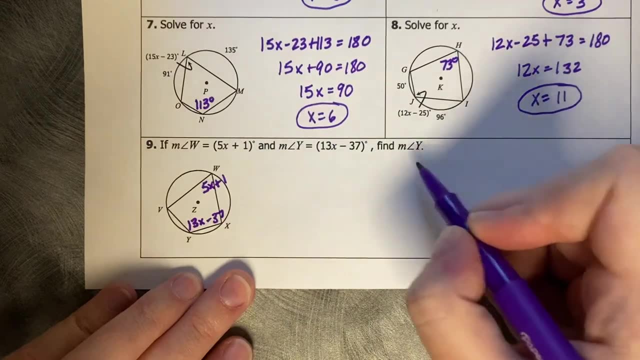 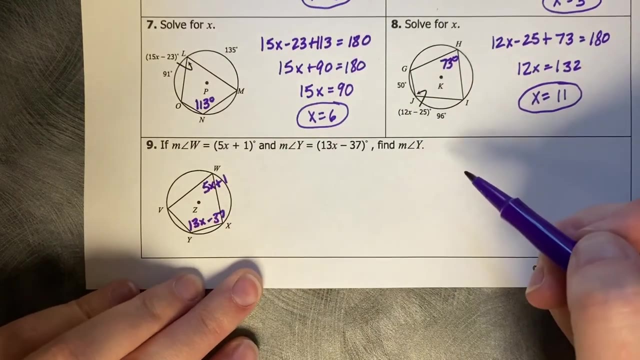 If the measure of angle W is 5X plus 1, and the measure of angle Y is 13X minus 37, find the measure of angle Y. So we know that those two angles together are supplementary. so we can set an equation up where we add these together and set it equal to 180. 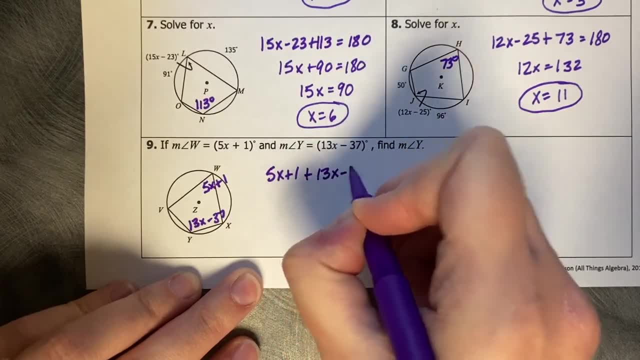 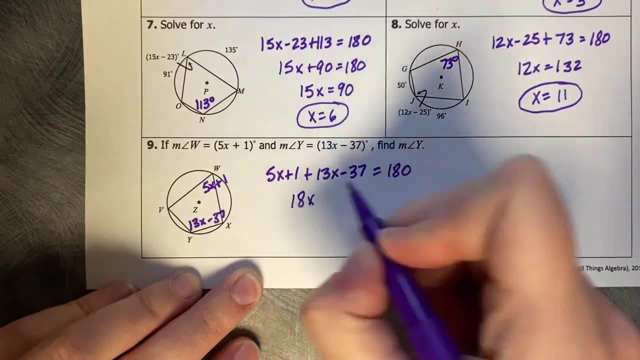 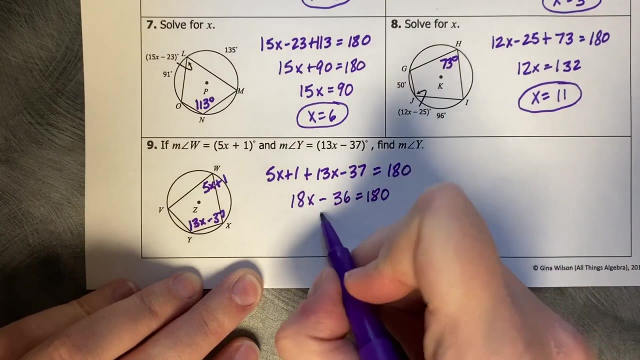 So 5X plus 1 plus 13X minus 37 equals 180.. 5 and 13 is 180.. 18X 1, and negative 37 is negative 36.. Plus 36, 18 equals 216..